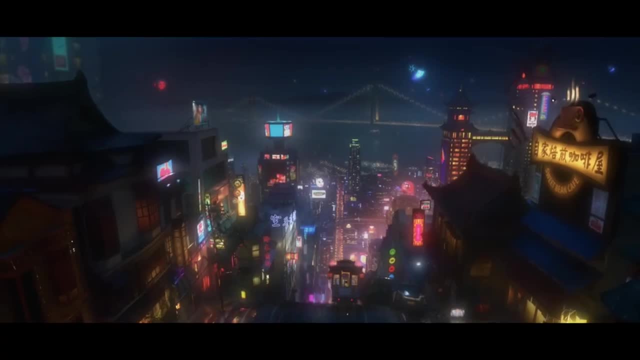 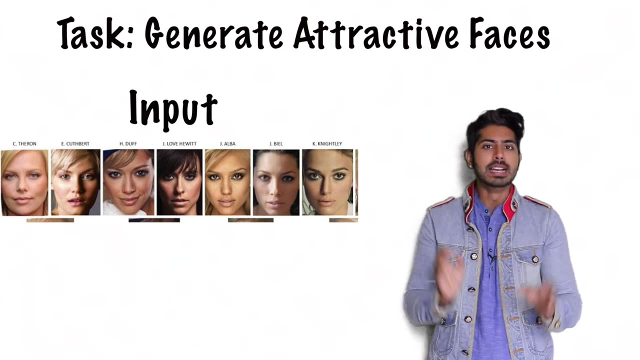 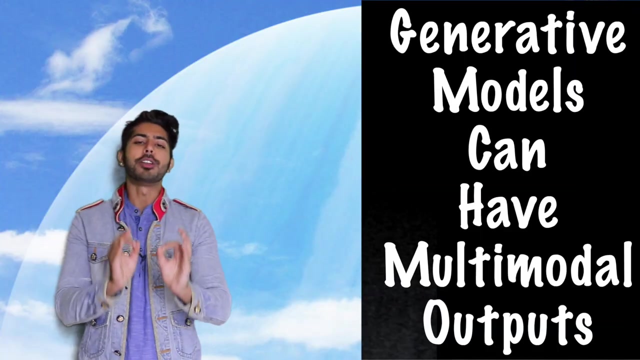 are thousands of different features or dimensions to this data. Can we generate an entirely new city from it? Atlantis is waiting. And what constitutes a good city? Sometimes, a single input corresponds to many different, correct answers, each of which is acceptable. 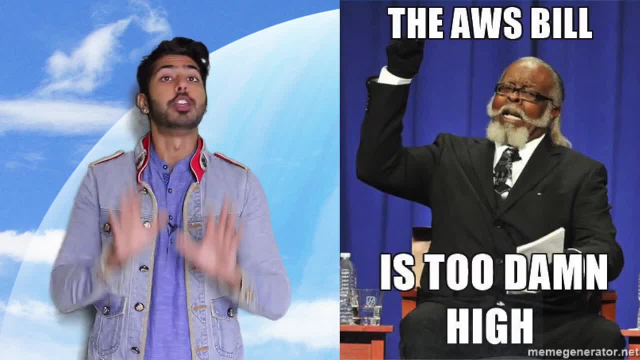 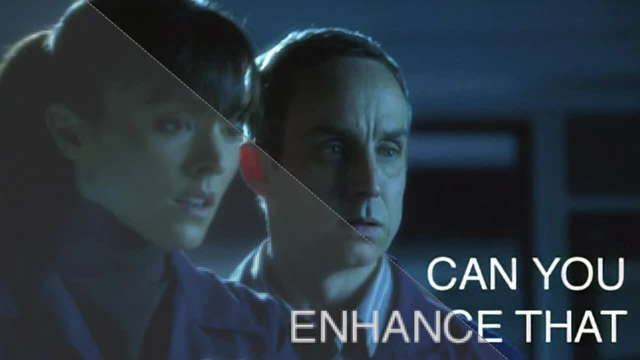 Generative models help us work with multimodal outputs like this. There's been so much activity centered around GANs lately. they've been used for a number of reasons. For example, they've been used to convert low-res images into crisp high-res images, convert hand-drawn. 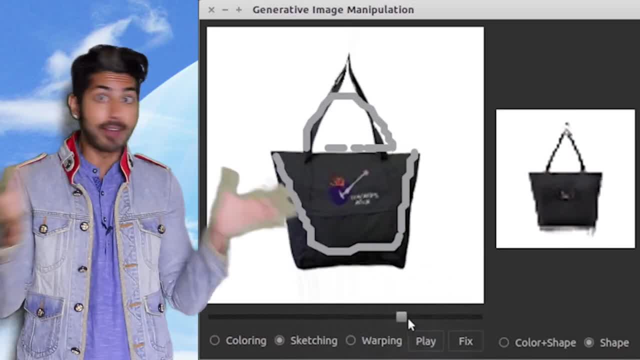 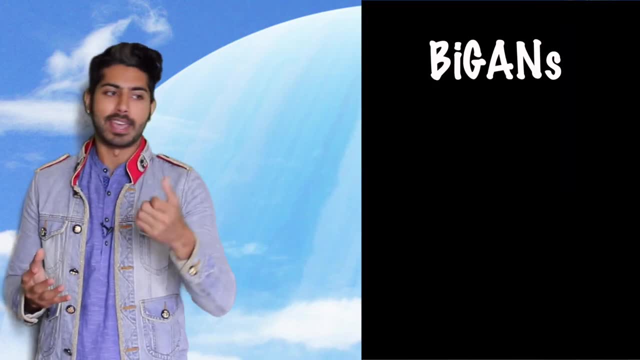 sketches into photorealistic images and to generate everything from fashion styles to new product categories. Apple- you should probably take a look into that last one. Buy GANs, Cycle GANs, WGANs- There's a lot. 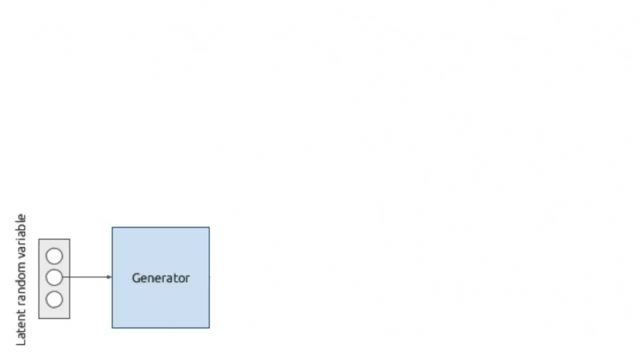 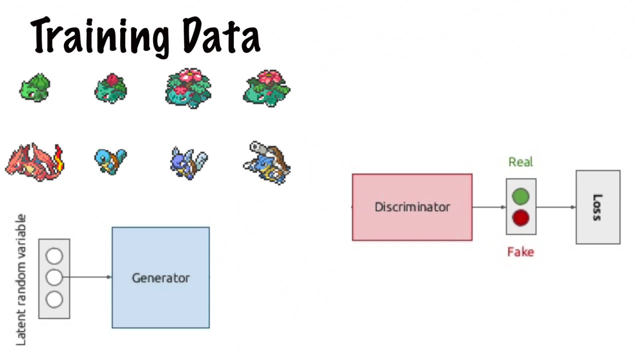 So the basic idea here is that we have two neural nets. One is called the generator G and the other is called the discriminator D. We've got some dataset- let's say it's a collection of Pokemon- And we want to generate new images from this dataset. that means entirely new Pokemon. 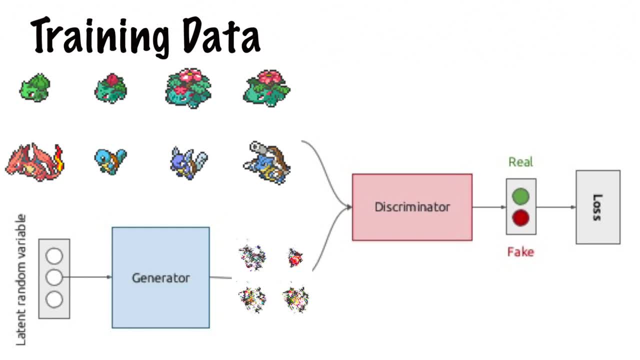 that have similar attributes to those in our training data. The generator's job is to try to create fake Pokemon that look really similar to our training Pokemon Ugh. The discriminator's job is to classify the generated Pokemon as either real or fake. Think of G as a magician. 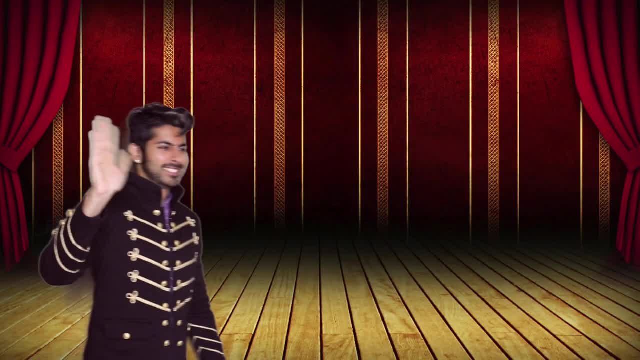 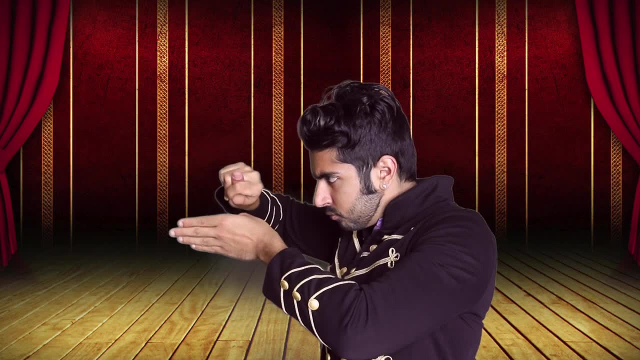 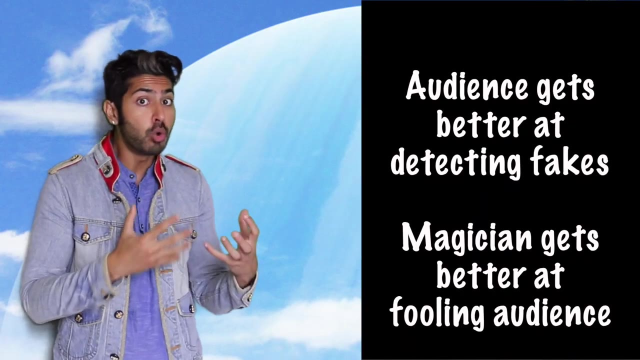 and D as his audience. The magician is constantly trying to make the audience believe that his Are real magic. the audience booze when it can tell that his tricks are fake and applaud when it can't tell the difference. They both improve and in the ideal case the magician gets so good that no matter. 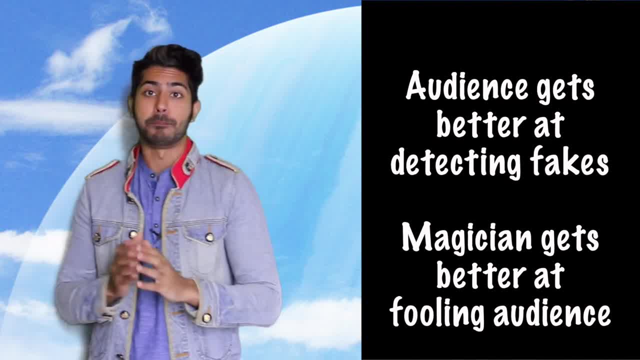 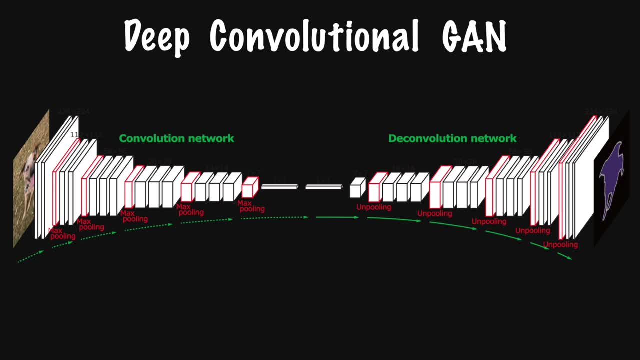 What he is able to fool his audience every time. the type of gain we'll use in this video is called a deep Convolutional Gann or DC Gann. this is because both D and G are deep convolutional neural nets, So the discriminator has several layers of what's called convolution and the generators got several layers of D convolution. 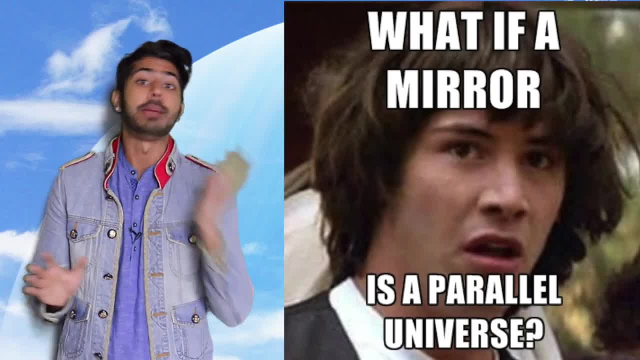 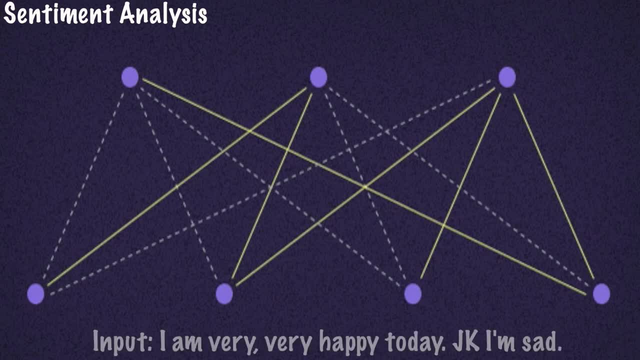 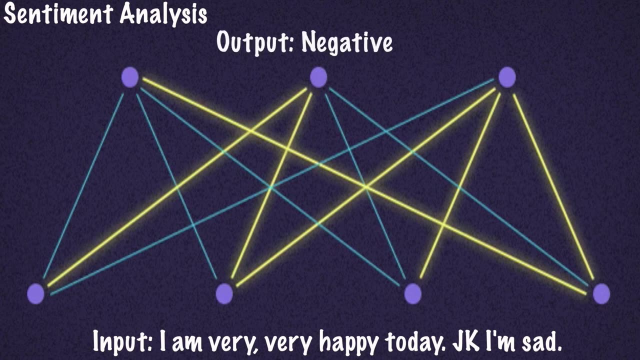 Convolution is literally impossible to understand in a parallel universe, but in this one It's pretty easy. Normally, neural net layers are fully connected, so all inputs are connected to all outputs. with many types of data. this makes sense. We want all parts of the input data to be able to contribute to all parts of the output prediction. 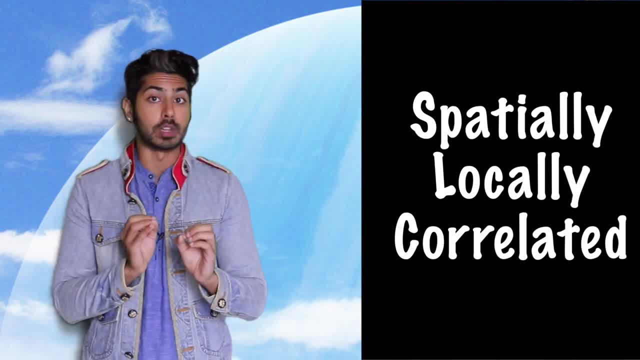 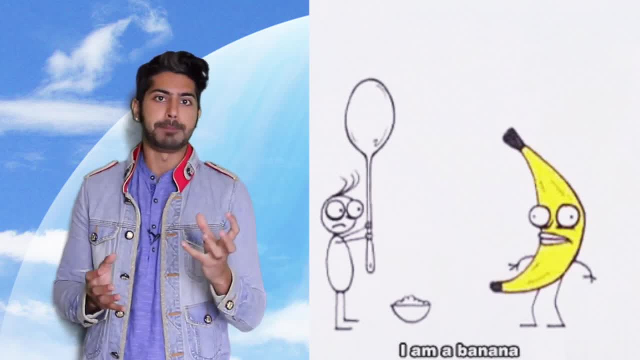 But images are considered Spatially locally correlated. that means if there's a banana in an image, It doesn't matter where it is in the image- It's still a banana. So we exploit that instead of connecting all of the input data or pixels to all output values. 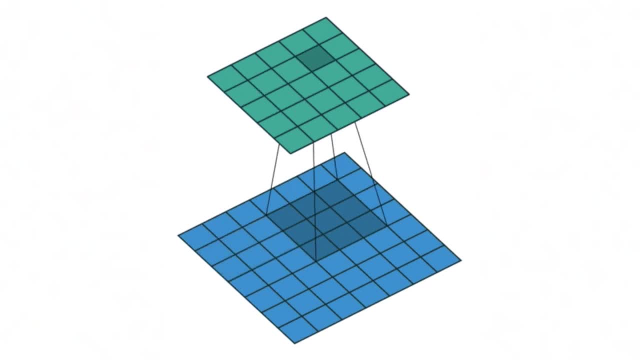 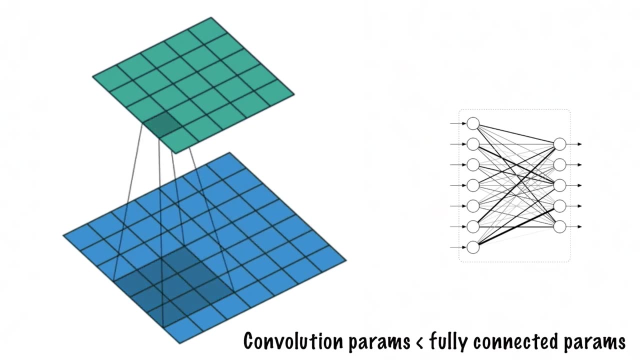 We use a much smaller filter that we slide across the picture like a flashlight, So that means much fewer parameters in a convolutional layer as opposed to a fully connected one. Let's look at our code. We're only going to use Keras to build our model pillow, helps us do image processing and 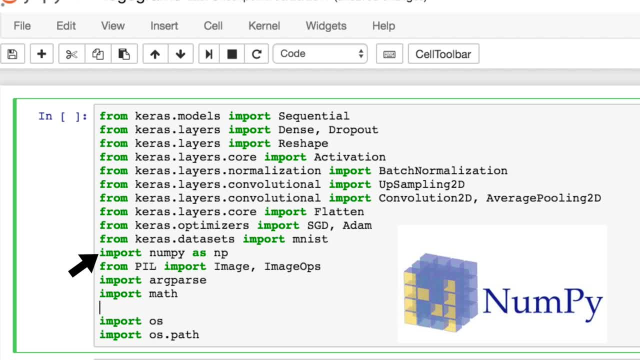 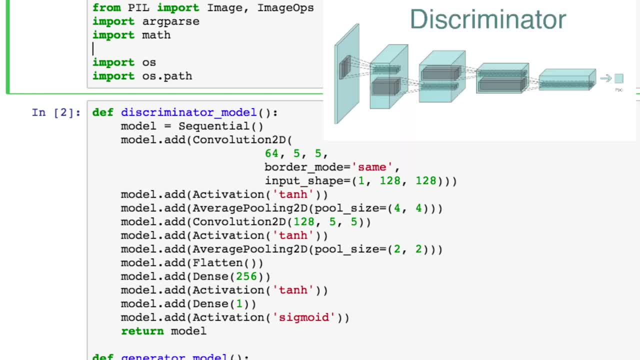 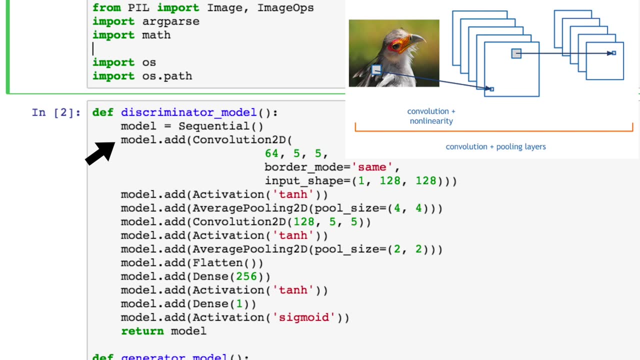 NumPy will help us perform some valuable reshaping operations on our images. Let's get started by first defining our discriminator. We'll give it its own function. It's going to be a linear stack of layers, So we'll define it as sequential and we'll start off with two convolutional blocks. that means a convolution to extract the feature map. 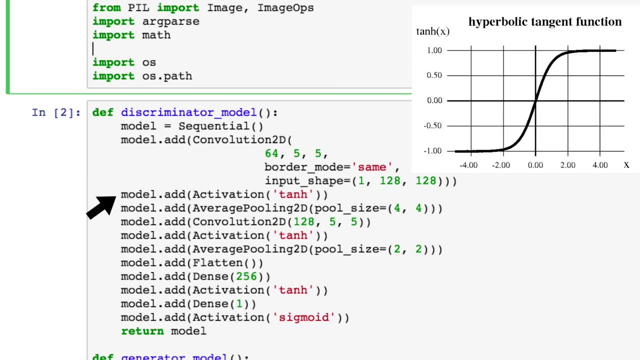 Followed by the tan H activation function to squash real numbers into a range between negative 1 and 1, Which lets our model learn more complex functions than just linear regression. then a pool Pooling. layer Pooling reduces the dimensionality of each feature map but retains the most relevant. 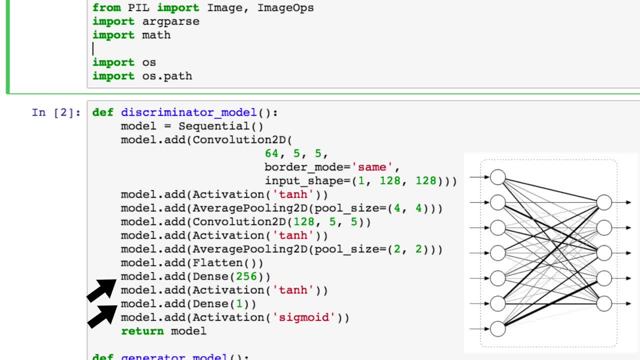 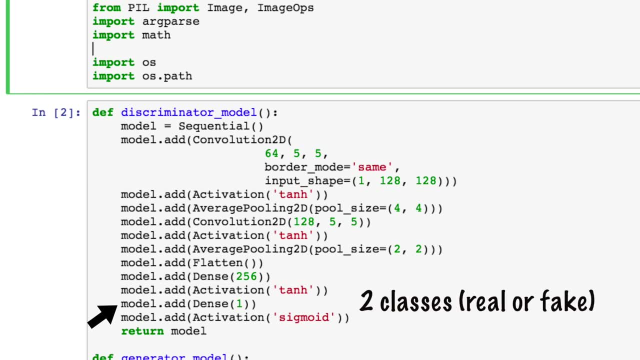 information. We'll flatten the feature map into one dimension, then apply two fully connected layers to it. The last dense layer outputs an n-dimensional vector, where n is the number of classes we have- so it would be 2 in our case- And by applying a sigmoid to it, it'll convert the data into probability values for each. 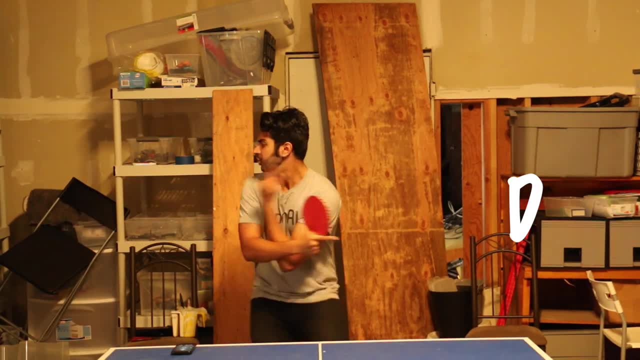 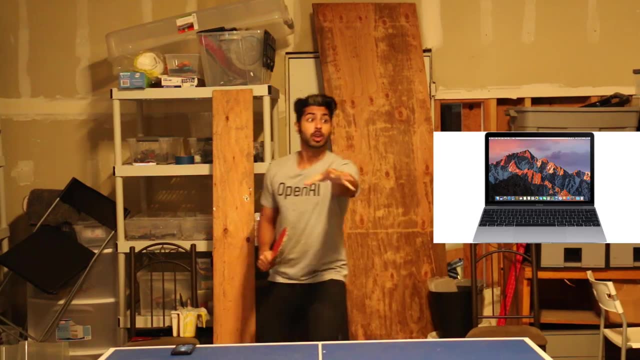 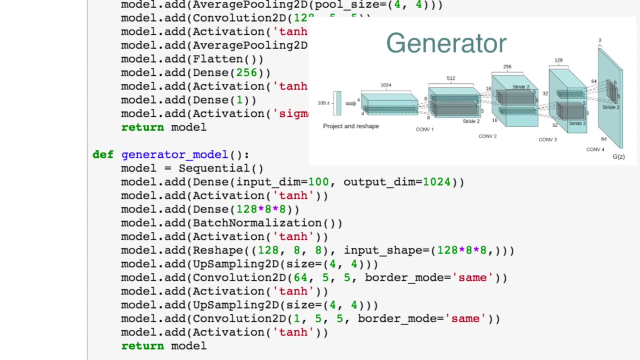 one. Next, we'll define our generator, which performs similar operations, but in the reverse order. Since it's fed random numbers as its input, it converts them into an image by first going through two fully connected layers with their own associated activation functions. 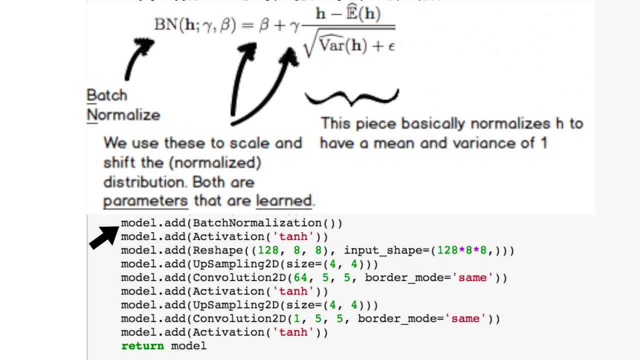 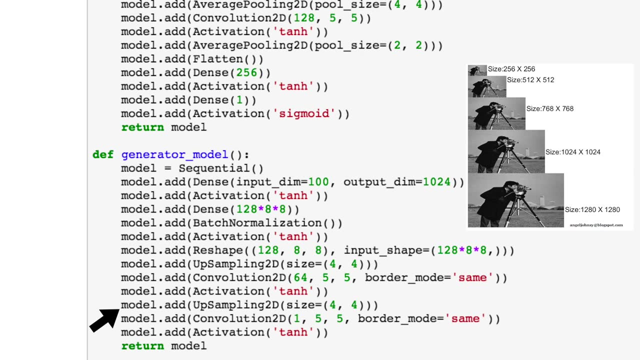 Batch normalization will apply a transformation that maintains the mean activation close to zero and the activation standard deviation close to one. This allows for faster learning and higher overall accuracy. Then we apply two convolutional blocks that will eventually output an image. Upsampling will convert our image into a higher resolution. 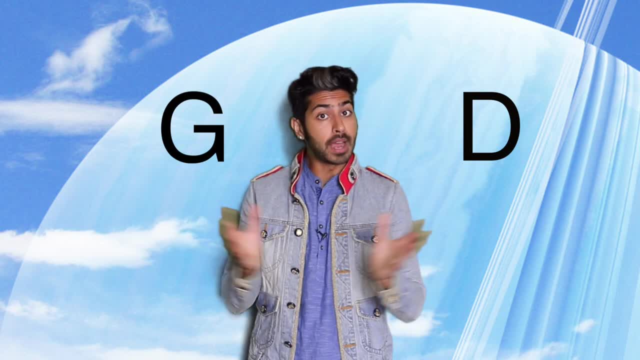 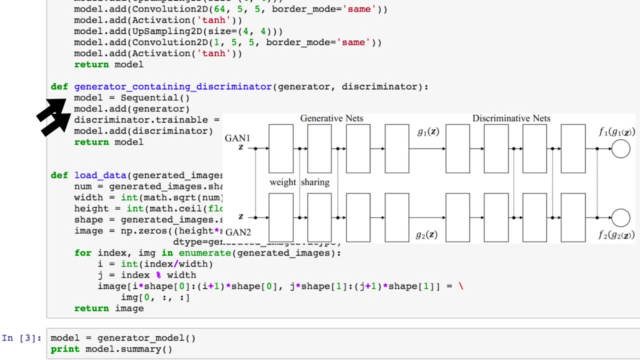 Now that we've defined models for both D and G, we can combine them to make a GAN pretty easily. with Keras, We can just reuse the same network objects we've already instantiated and they'll conveniently contain the same shared weights with the previously compiled models. 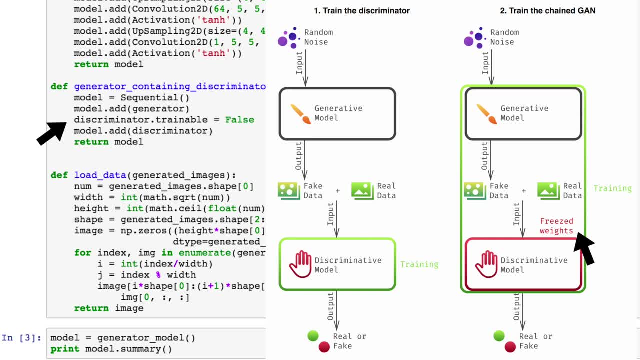 We're going to want to freeze weights in the discriminator part of the GAN when we back propagate the joint models. so we'll first set the Keras trainable flag to false for each element in this part of the network. We'll also define a loadData function which will form our images into vectors that we 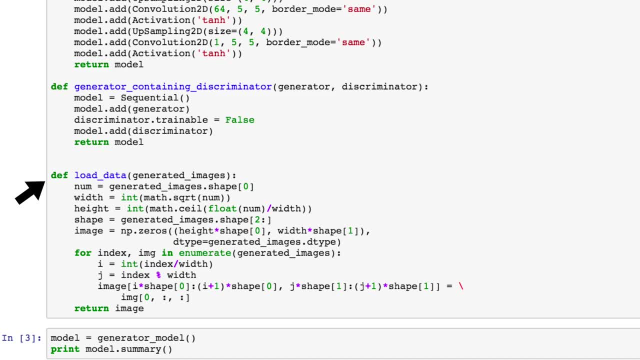 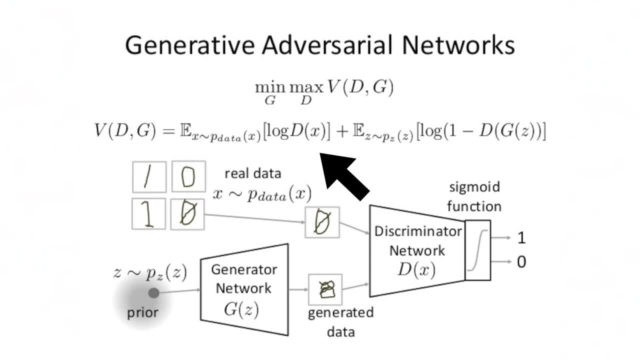 can feed to our model by making use of the image and numpy libraries. Okay, so how do we train this thing? The goal of training our discriminator is to maximize the amount of data that we're going to use for every image from the true data distribution and minimize the amount. 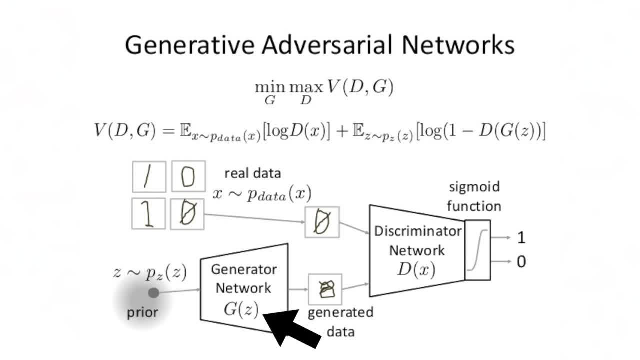 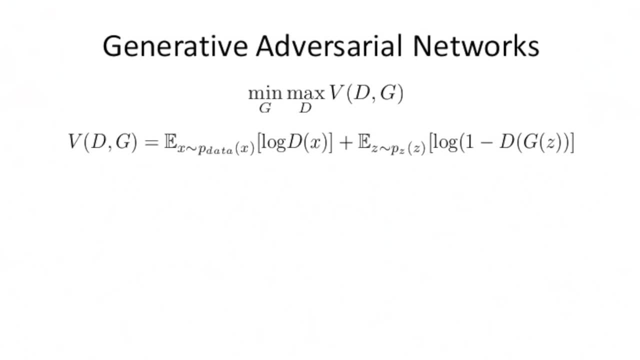 of data that we're going to use for every image, not from the true data distribution. The goal of training the generator G of Z is to create samples that fold D. We train both D and G by taking the gradients of this expression with respect to their parameters. 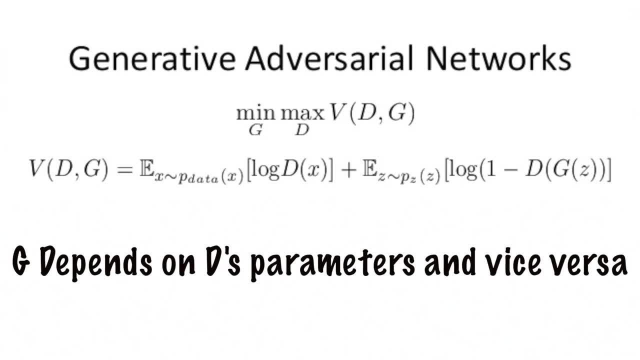 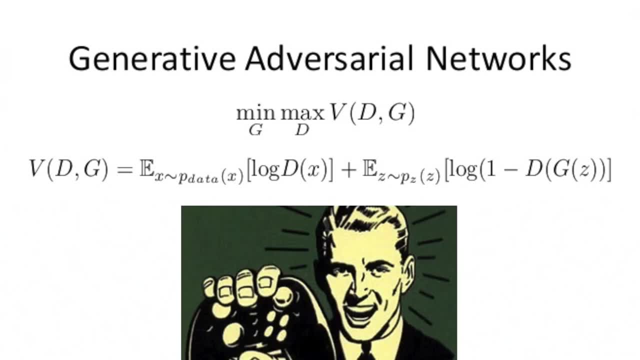 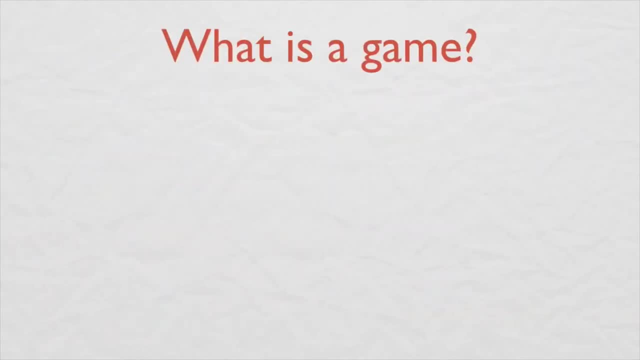 Because each player's cost depends on the other player's parameters, but each player cannot control the other player's parameters. this scenario is most straightforward to describe as a game rather than an optimization problem, specifically a minimax game. Minimax is a strategy of always minimizing the maximum possible loss which can result. 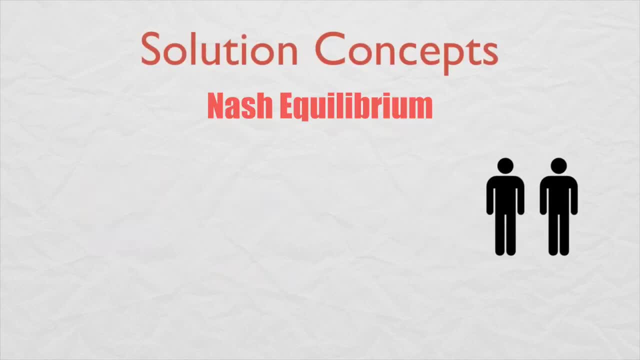 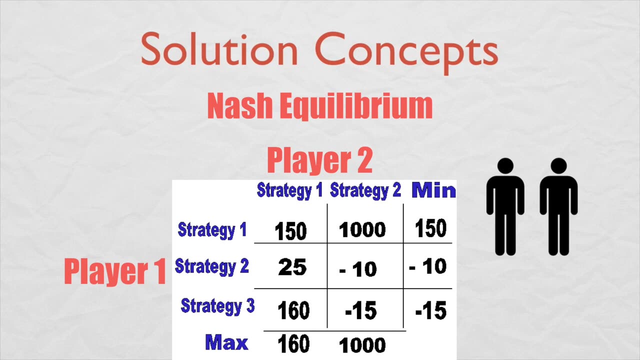 from a choice that a player makes, and the Nash equilibrium is where the optimal outcome of a game is one where no player has an incentive to deviate from his chosen strategy after considering an opponent's choice. So the way we train GANs is to find the Nash equilibrium of a minimax game between G and 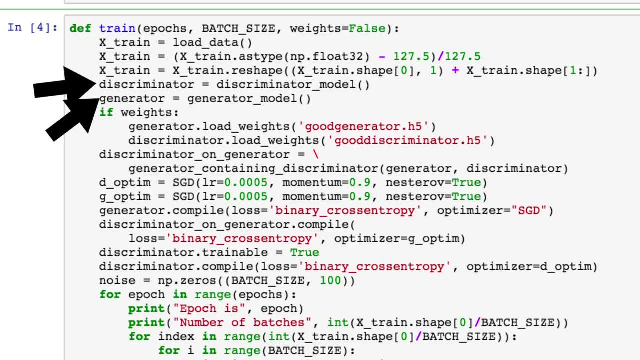 D, We load our data and initialize both of our models in our train function. Then we'll combine them both and initialize stochastic gradient descent optimizers. for both of them. We'll define a loss function, binary cross entropy, then perform the set of steps outlined. 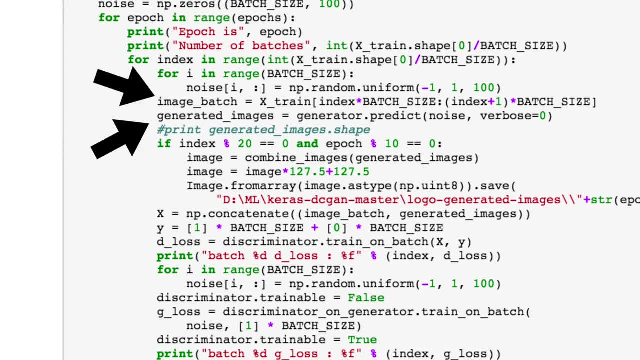 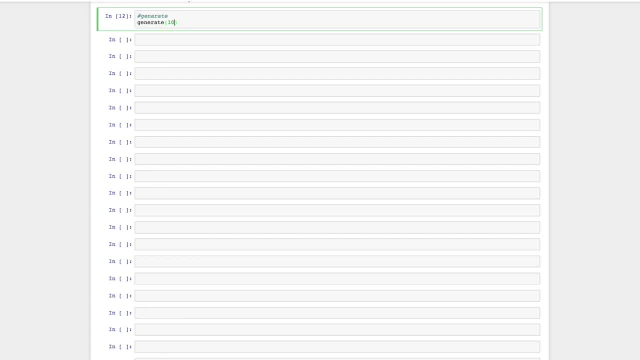 in the paper. For every time step we sample data from both distributions, then update D using our gradients, Then we update G using our gradients. Once we're done training, we can generate some images from G and we'll see that they.